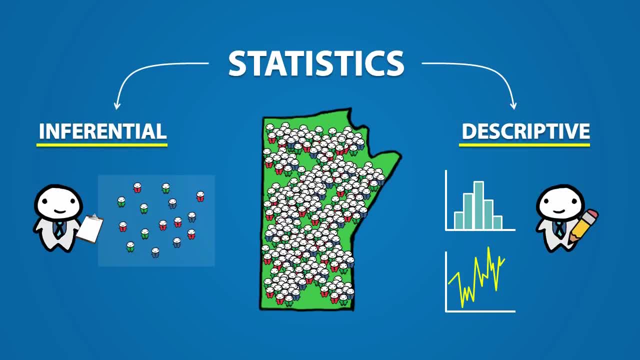 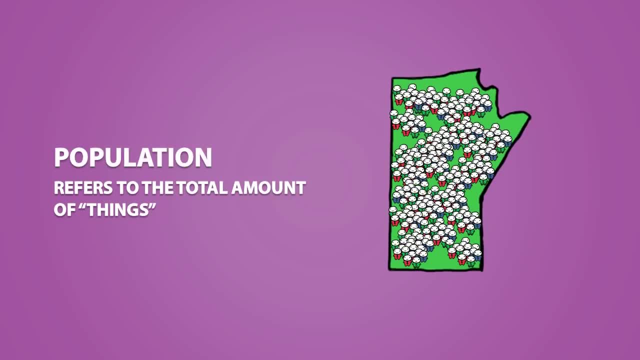 deals with inferential statistics. In order to understand statistics, you'll first have to know some basic definitions. A population refers to the total amount of things. I say things because a population can refer to almost anything. This can refer to the total amount. 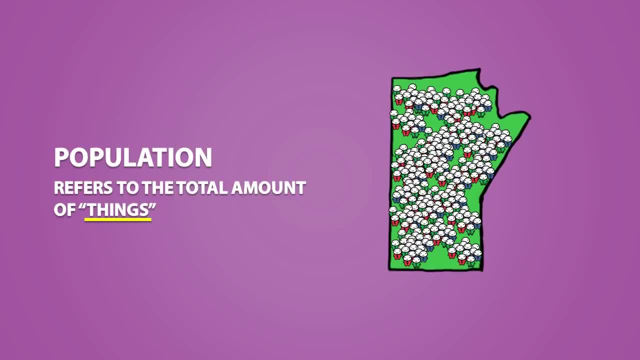 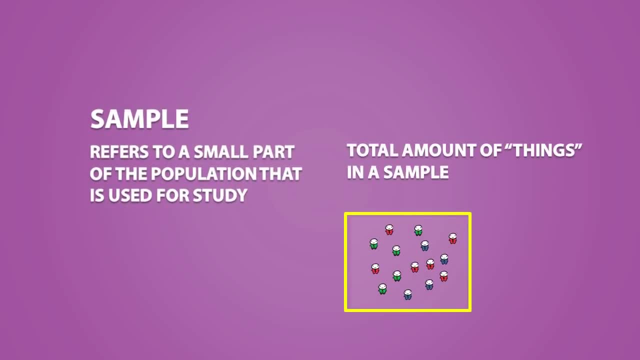 of people, cats, vehicles, houses and so on. Now, a sample refers to a small part of the population that is used for study, and the total amount of things in a sample is called the sample size. In statistics, what we examine is a variable. It is what we are. 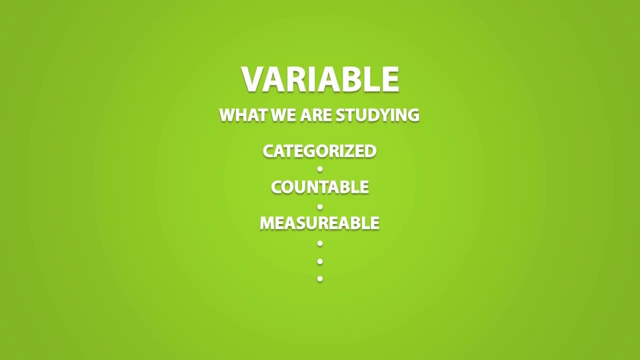 studying and it can be measurable, countable and categorized. When we talked about how people can have different heights, weights and hair color, these are all variables. Variables represent a characteristic of what we are trying to study and they can vary among different 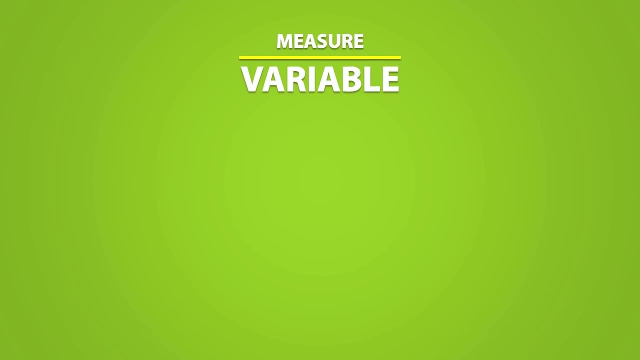 individuals. When we measure a variable, our data can come into two different forms. There is categorical data and there is quantitative data. Quantitative data refers to data that is measured in numbers. It deals with numbers that make sense to perform arithmetic calculations. 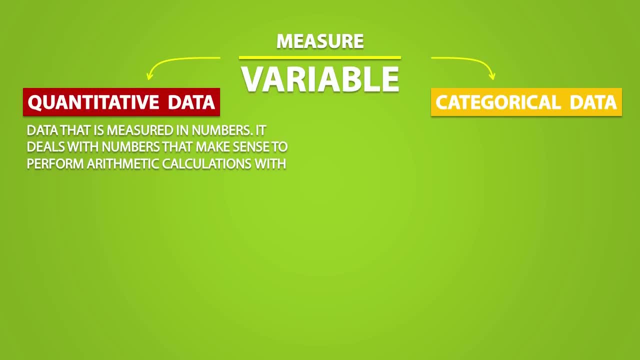 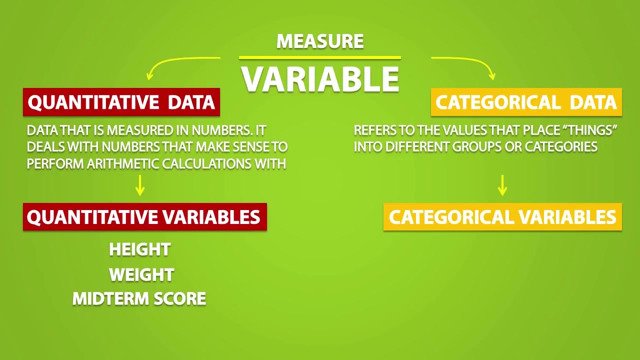 with like calculating an average. Quantitative data comes from quantitative variables. Examples include height, weight and midterm score. On the other hand, categorical data refers to values that place things into different groups or categories. Categorical data comes from categorical variables. Examples include hair color, type of cat and letter grade. 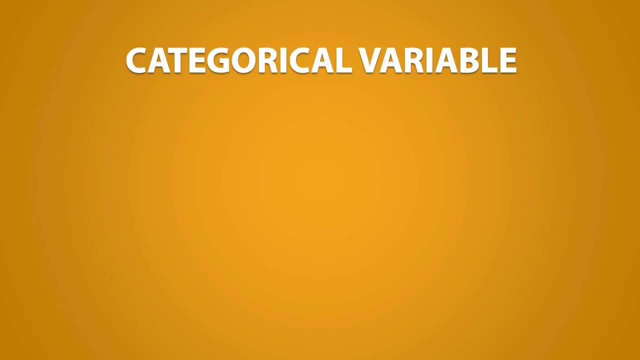 There are actually two types of categorical variables. There is categorical and ordinal, and categorical and nominal. Something is said to be categorical and ordinal if there is a logical ordering to the values of a categorical variable. A good example of this would be letter grade. We can logically order the values of this categorical variable from high to low. 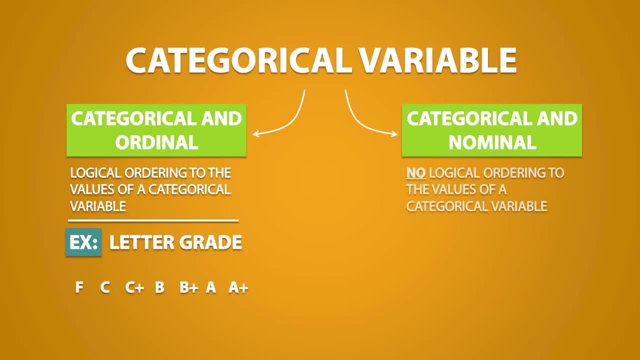 or from low to high. Now, something is said to be categorical and nominal. if there is no logical ordering to the values of a categorical variable, An example of this would be hair color. Depending on our sample, we could have people with red hair, blonde hair, brown hair or 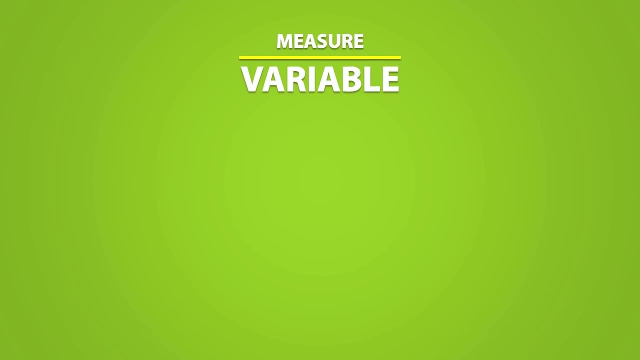 individuals. When we measure a variable, our data can come into two different forms. There is categorical data and there is quantitative data. Quantitative data refers to data that is measured in numbers. It deals with numbers that make sense to perform arithmetic calculations. 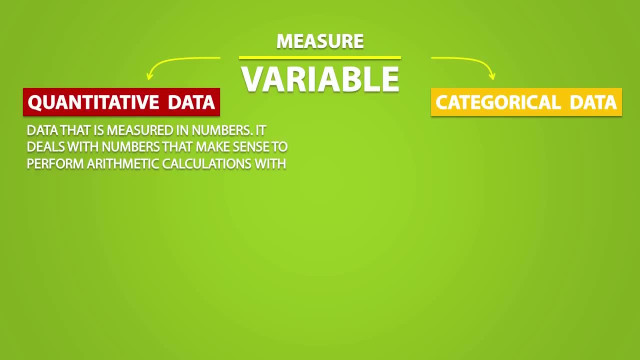 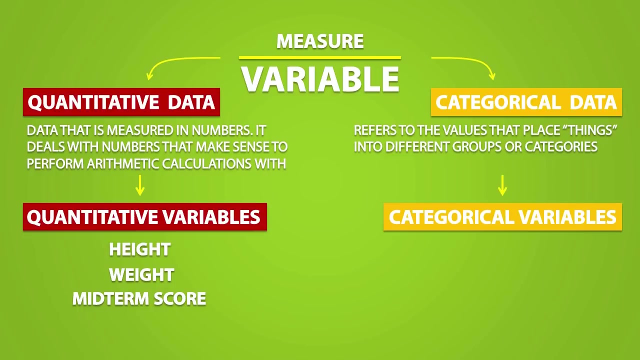 with like calculating an average. Quantitative data comes from quantitative variables. Examples include height, weight and midterm score. On the other hand, categorical data refers to values that place things into different groups or categories. Categorical data comes from categorical variables. Examples include hair color, type of cat and letter grade. 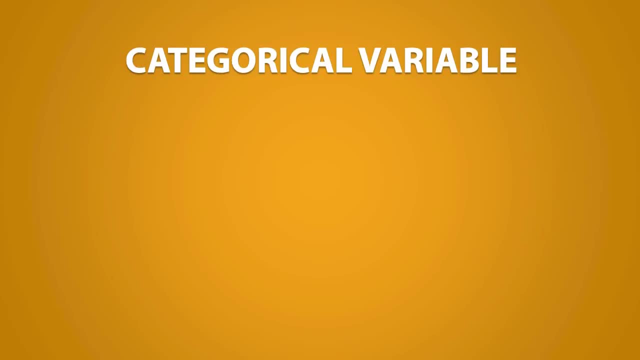 There are actually two types of categorical variables. There is categorical and ordinal, and categorical and nominal. Something is said to be categorical and ordinal if there is a logical ordering to the values of a categorical variable. A good example of this would be letter grade. We can logically order the values of this categorical variable from high to low. 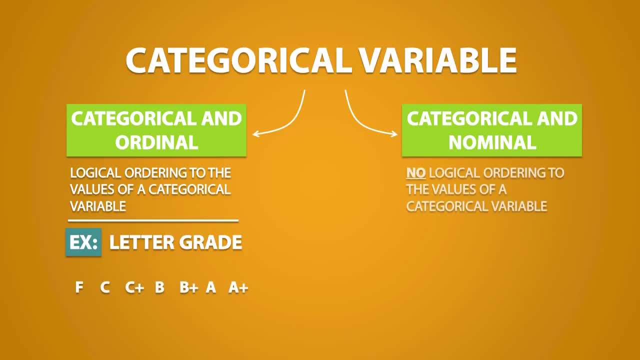 or from low to high. Let's see what we can do Now. something is said to be categorical and nominal if there is no logical ordering to the values of a categorical variable. An example of this would be hair color. Depending on our sample, we could have people with red hair, blonde hair, brown hair or even blue. 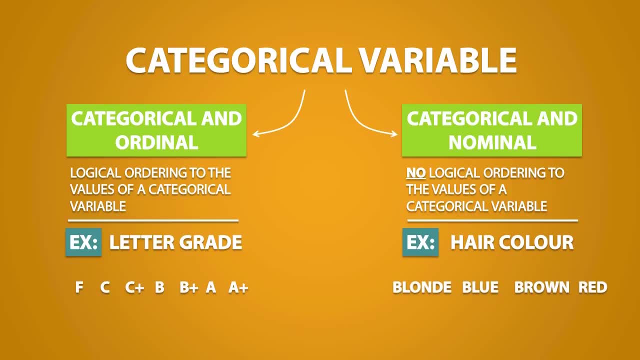 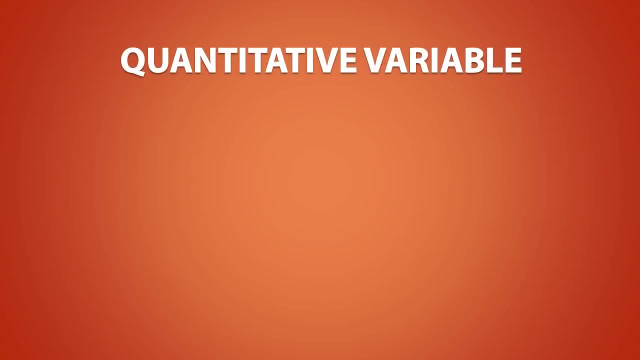 hair. Although we can arrange these values in alphabetical order, there is no logical ordering. with respect to the actual values itself, There are also two types of quantitative variables: There is discrete and continuous. There is discrete and continuous. There are also two types of quantitative variables. There is. 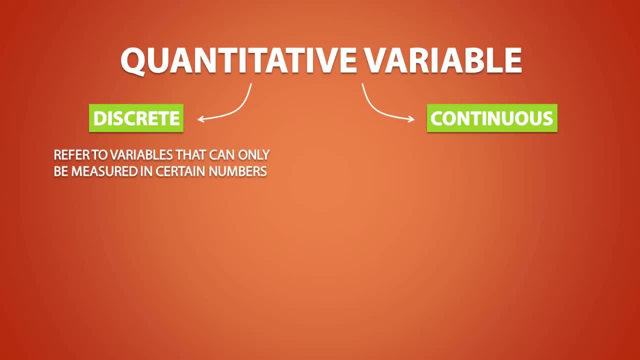 discrete and continuous. Discrete variables refer to variables that can only be measured in certain numbers. An example of this is the number of pets you own. You can own 0 pets, 1 pet, 2 pets or even 30 pets, but it's impossible for us to own 2.7 pets. 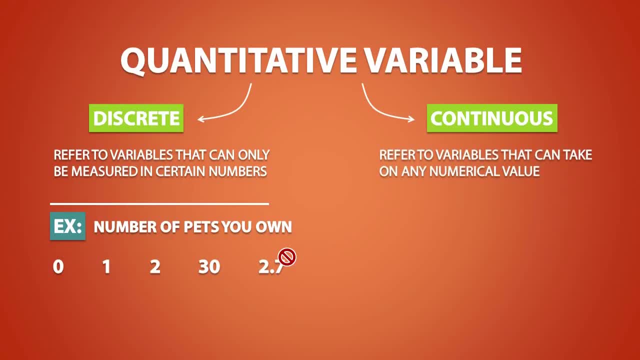 In contrast, continuous variables refer to variables that can take on any numerical value. An example of this would be weight. Someone can weigh 105 pounds, 185 pounds or even 170.683 pounds. We can measure this variable in as many decimal places as we want, which.